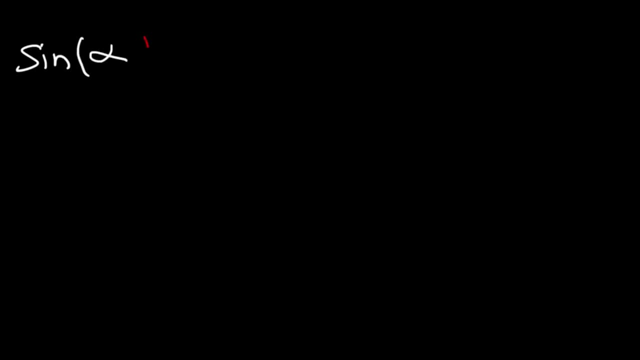 formula for sine Sine alpha plus or minus beta. that's equal to sine alpha cosine beta plus or minus cosine alpha sine beta. So notice that the sine doesn't change. So if you use the positive sign on top, then you should use the positive sign on top as well. on the right. 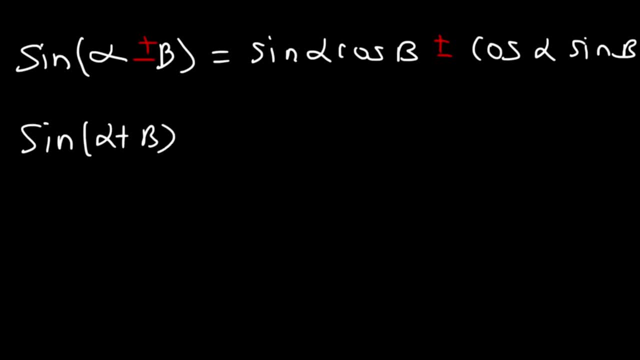 So therefore sine alpha plus beta is equal to sine alpha cosine beta plus cosine alpha sine beta, And so this was a minus sign. then you would change it to a minus sign Now. the only other formula need to know is tangent. It's tangent alpha plus or minus beta is. 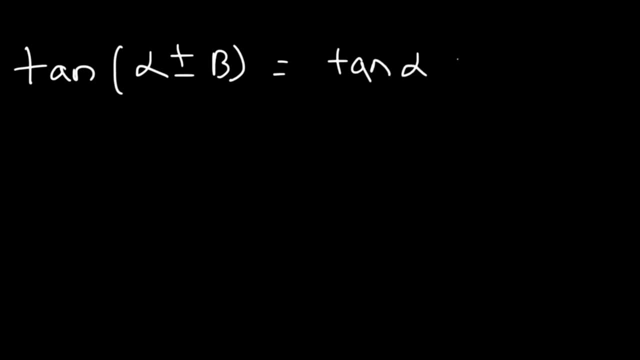 equal to tangent petals alpha plus or minus tan beta divided by 1 minus plus tan alpha tan beta. so if we want to use the bottom sign, let's say if it's negative here, then it's going to be negative on top and positive on the bottom. so just keep that in mind. now, 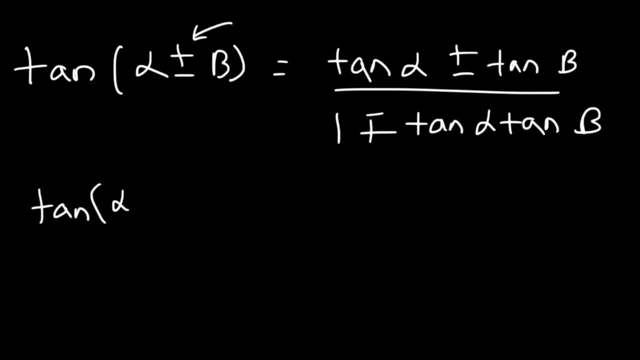 let's say if we want to use the upper side, let's say if it's alpha plus beta, so if we're using the positive sign, we need to use the upper sign in both cases. so tangent alpha plus beta, for example, it will be tangent alpha plus tangent. 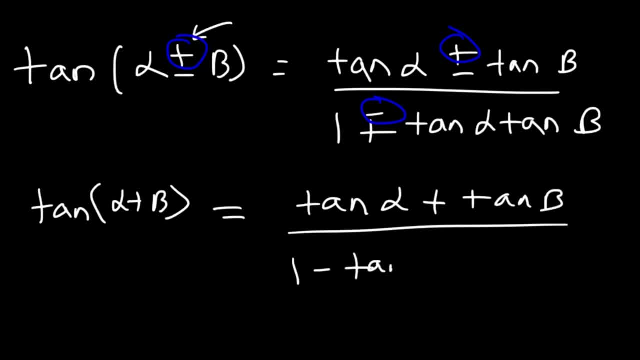 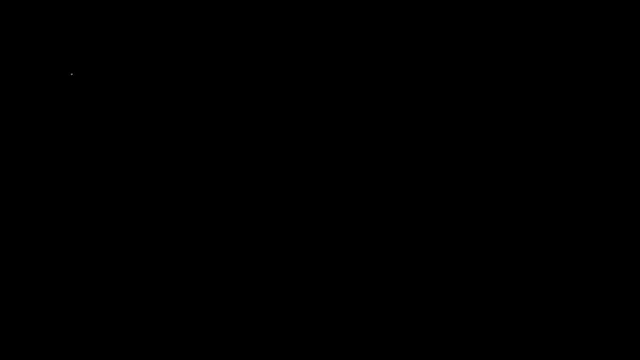 beta divided by 1 minus tangent alpha times tangent beta. so make sure you know these formulas. now how can we use the sum and difference formulas to evaluate sine of 15 degrees? so first we need to find two angles that either add or subtract to 15, two common 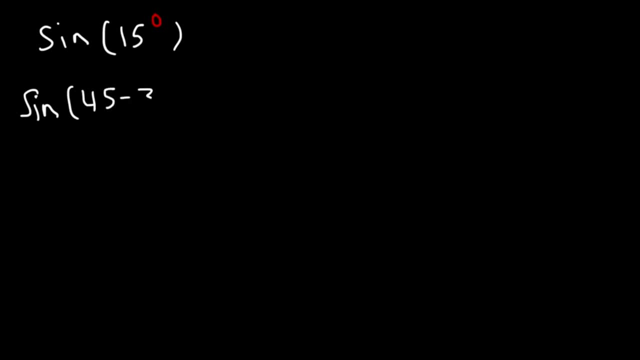 angles that we know on a unit circle are 45 and 30. 45 minus 30 is 15. so we're going to use the formula: sine alpha minus beta is equal to sine alpha cosine, beta minus cosine, alpha sine beta. So, as we can see, alpha is 45 and beta is 30. So sine 45 minus 30,. 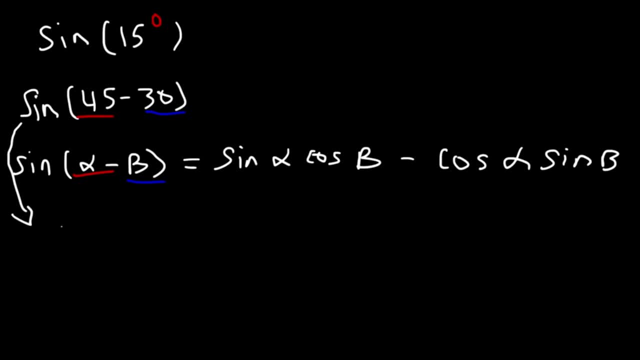 I'm going to put it over here. that's equal to sine 45, cosine 30 minus cosine 45 times sine 30. Now we know that sine 45 is the square root of 2 over 2.. Cosine 30 is the square root of 3 over 2.. 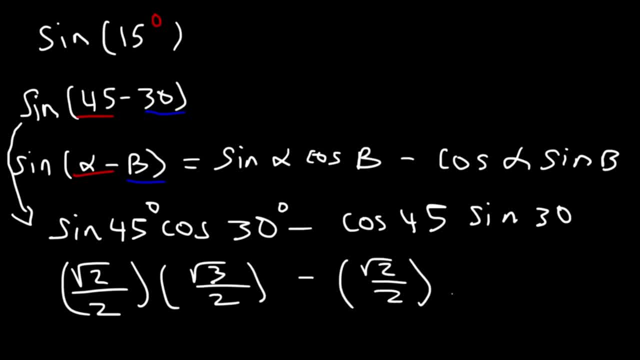 Cosine 45 is the same as sine 45, and sine 30 is 1 half. Now let's multiply the square root of 2 times the square root of 3, and that's equal to the square root of 6, and 2 times 3.. 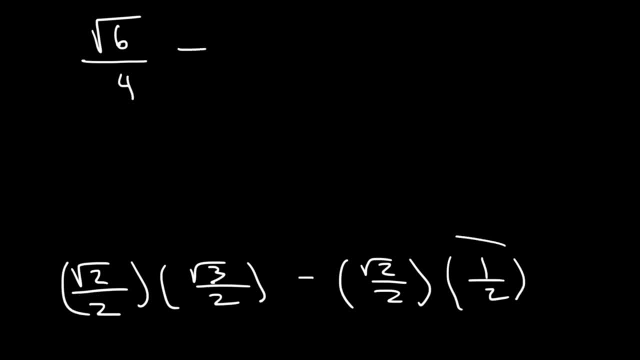 And here we have the square root of 2 times 1, which is simply square root 2 over 4.. So we can combine this as a single fraction, if we want to. So square root 6 minus square root 2 divided by 4 is equal to sine of 15 degrees. Now let's try another example: Sine 105.. So go ahead. 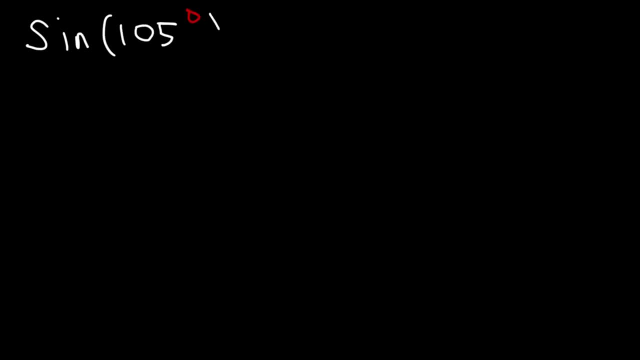 and use the sum and difference formula To find the exact value of sine 105.. Now the first thing we need to do is find two common angles on a unit circle that adds up to 105.. So this is 60 plus 45. So this time we're going to 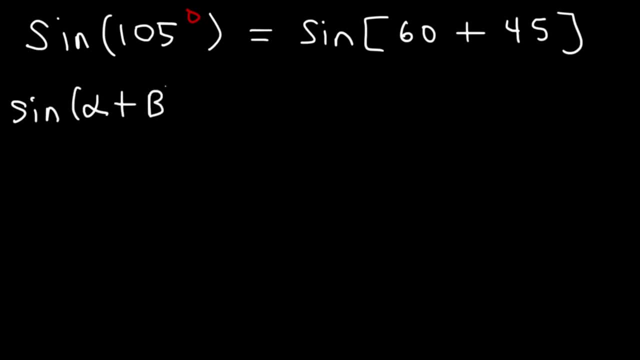 use the formula sine alpha plus beta is equal to sine alpha, cosine beta plus cosine alpha times sine beta. So alpha 60 beta is 45.. So this is going to be sine 60- cosine 45 plus cosine 60 times sine 45.. Sine 60 is equal to the square root of 3 over 2.. Cosine 45: 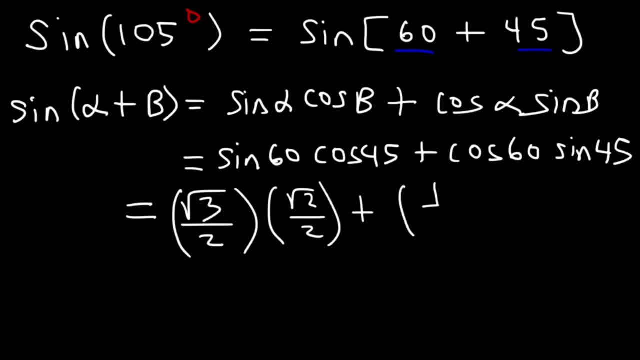 is the square root of 2 over 2.. Cosine 60 is one half And sine 45 is equal to the square root of 2 over 2.. So now what we have is the square root of 6 over 4 plus the square root of 2 over 4.. So the 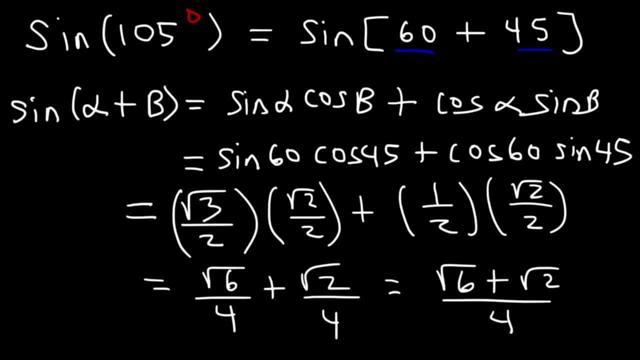 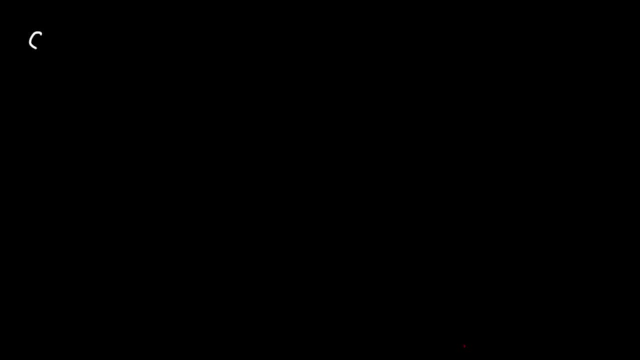 final answer is root 6 plus root 2 over 4.. And so that is equal to sine of 105 degrees. So that's how you can use the sum and difference formulas to evaluate. So in trigonometric expressions- Here's another one that we can try: Cosine 2 pi divided by 3 minus pi over 6.. 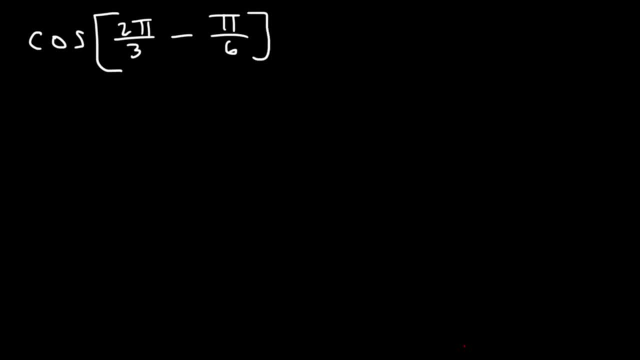 So use the sum and difference formulas of cosine to evaluate this one. So we need to use the difference one Alpha minus beta. So this is equal to cosine alpha times cosine beta. And because we have a minus here, we need to change the sign, So it's going to be plus. 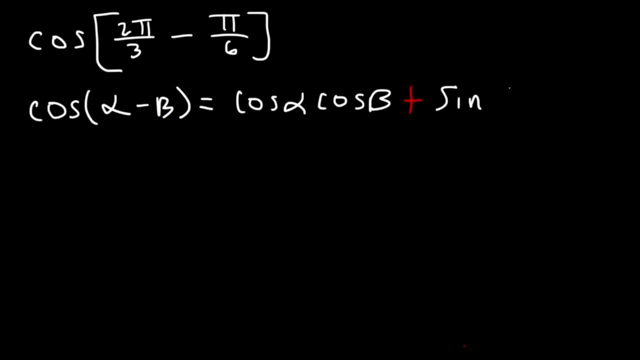 sine alpha, sine beta. Now we can see that alpha is 2 pi over 3 and beta is pi over 6.. So this is equal to cosine 2 pi divided by 3 times cosine pi over 6, plus cosine 2 pi divided by 3.. So this is: 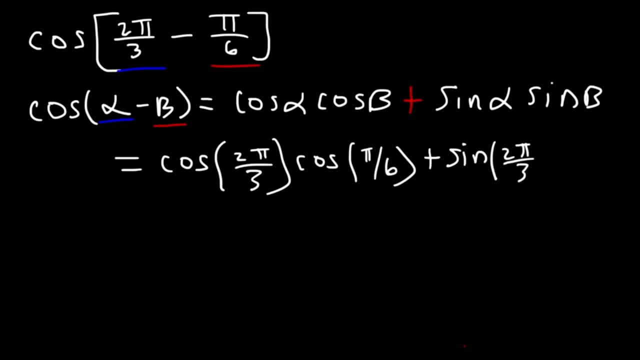 equal to sine of 2 pi over 3 times sine pi over 6.. Pi over 6 is 30 degrees. 2 pi over 3, that's 120.. Cosine 120, that's in quadrant 2, so it's negative. That's equal to negative 1 half. 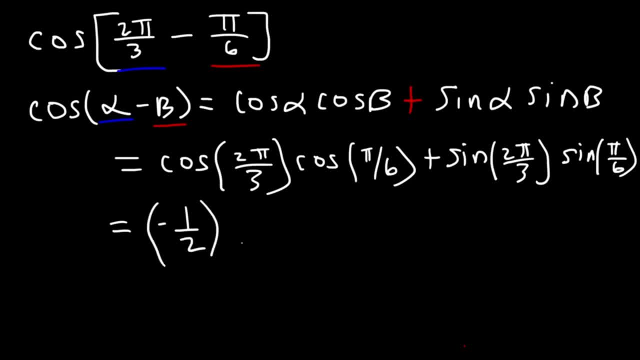 The reference angle is pi over 3, which is 60.. Cosine of 60 is 1 half. Cosine 30 is root 3 over 2.. Sine 120 is root 3 over 2. And sine 30 is simply 1 half. So this is negative square root 3 over 4. 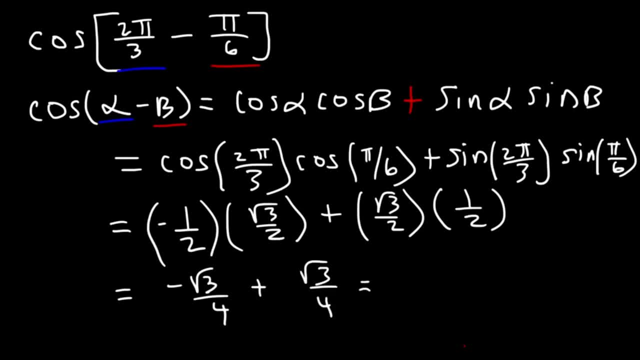 plus positive square root, 3 over 4, which really is 0. And it makes sense. This is 120 minus 30. So that's cosine of 90.. At 90 degrees on the y-axis, the independent éléments pass through is 0. And so we get this, which is 0. And then we get y-axis, which is 9.. So 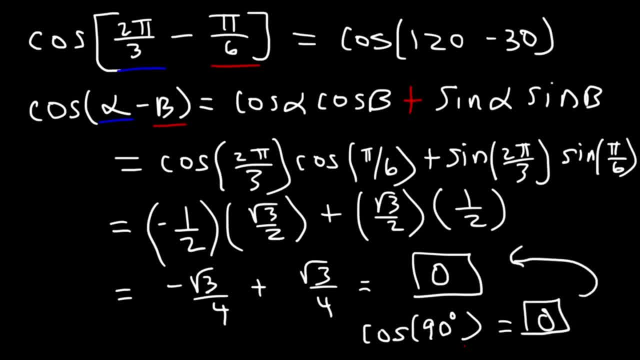 Shade of 90 degrees Degrees on the y-axis, So that's cosine of 90.. At 90 degrees on the y-axis, The x value is 0, and so that's it for this problem. Let's work on this example. 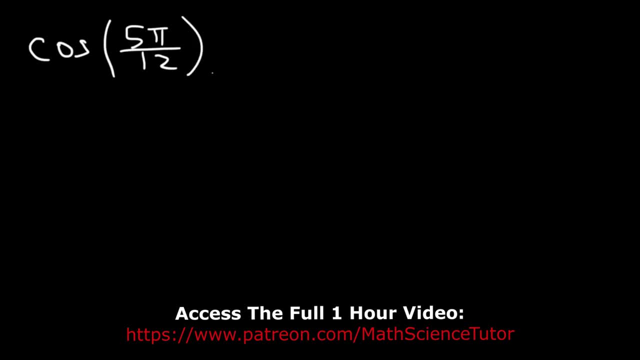 Cosine, 5 pi over 12.. Go ahead and evaluate it Now. 5 pi over 12 is not on a unit circle, so we need to use the sum and difference formulas of cosine. But first let's convert 5 pi over 12 into degrees. 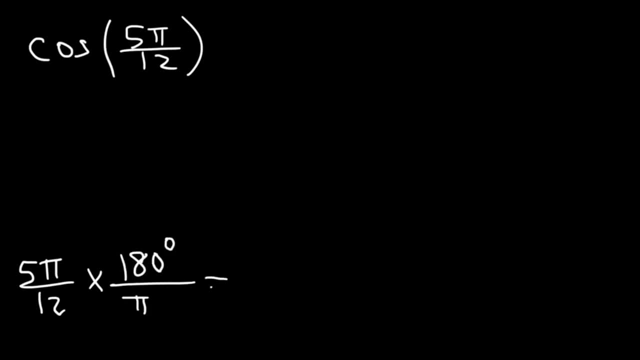 So let's multiply it by 180 divided by pi, So we can cancel pi. 180 is 18 times 10, and 12 is 6 times 2.. I'm going to break down 18 into 6 times 3, and 10. I'm going to write it as 5 times 2.. 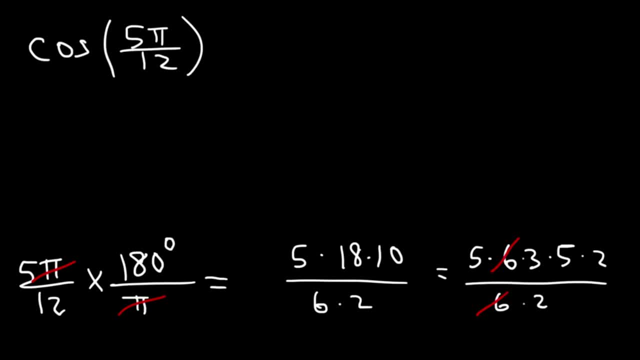 So we could cancel a 6, and we could cancel a 2.. 5 times 5 is 25.. 25 times 3 is 75. So this is the same as cosine 75 degrees. So we need to use this formula. 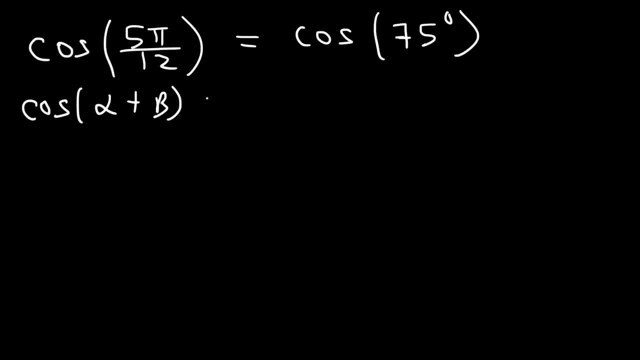 Cosine alpha plus beta is equal to cosine alpha- cosine beta. and then, since we have a plus sign, we're going to flip it and make it minus, So it's minus sine alpha times sine beta. Two angles that add up to 75 are 45 and 30. 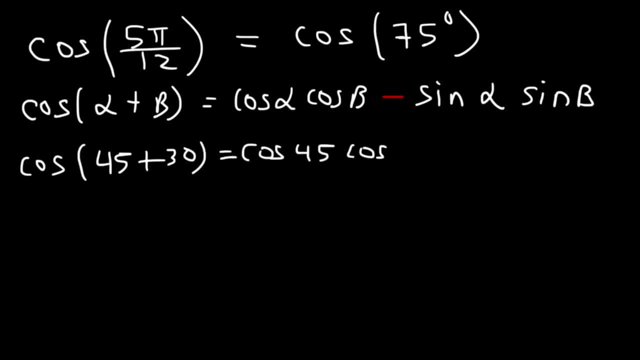 So this is equal to cosine 45,, cosine 30, minus sine 45 times sine 30. So cosine 45,, that's equal to the square root of 2 divided by 2.. Cosine 30 is the square root of 3 over 2.. 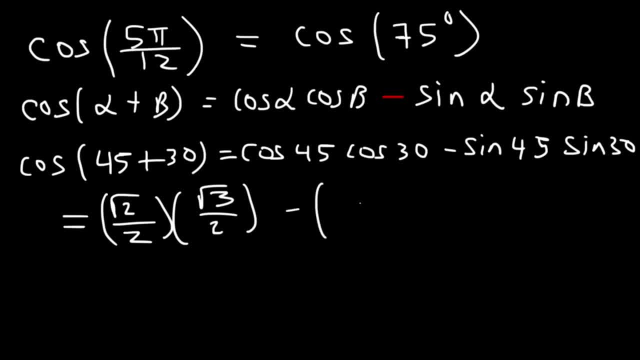 So cosine 45 is the square root of 2 divided by 2. Cosine 30 is the square root of 3 over 2. Cosine 45 is the square root of 3 over 3. Sine 45, that's root 2 over 2.. 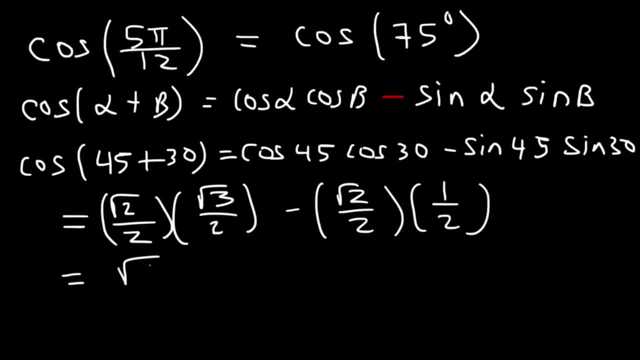 Sine 30 is one half. So this is going to be equal to the square root of 6 over 4 minus the square root of 2 over 4, which is root 6 minus root 2 over 4.. So this is the final answer. 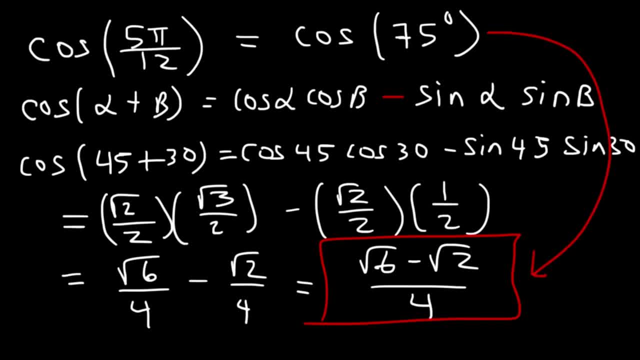 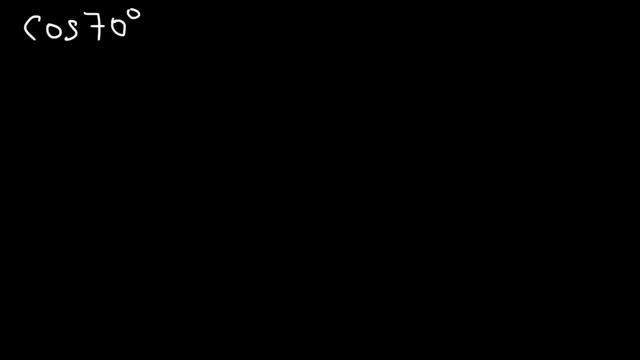 Cosine 75 or cosine 5, pi over 12 is equal to that. Find the exact value of the expression. Find the exact value of the expression: Cosine of 70 degrees multiplied by cosine of 40 plus sine, 70 times sine 40.. 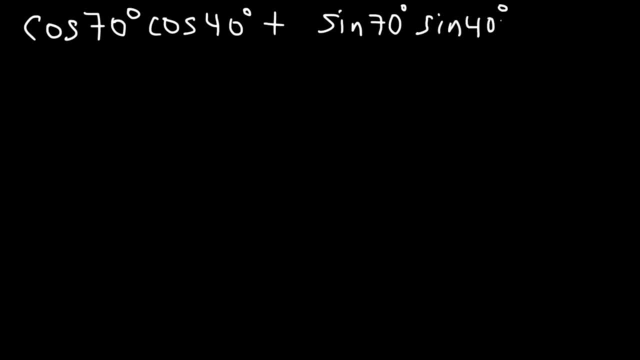 So we can't just type it in the calculator And we don't know the value of cosine 70. So what should we do in this case? You need to identify the proper formula. So we have cosine times, cosine plus sine times, sine. 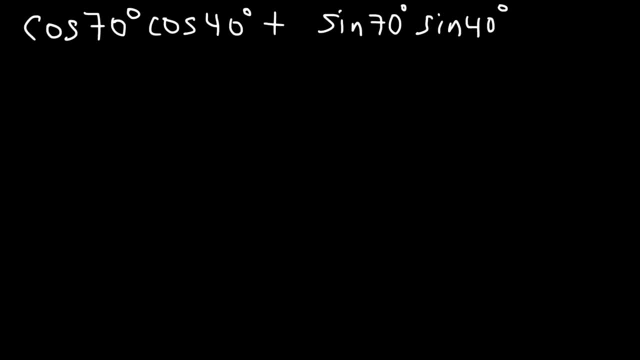 This is associated with the sum and difference formulas of cosine. Now is it cosine alpha plus beta or cosine alpha minus beta? With cosine you got to change the sign, So we need to use this formula: Cosine alpha minus beta. is cosine alpha, cosine beta plus sine, alpha sine beta. 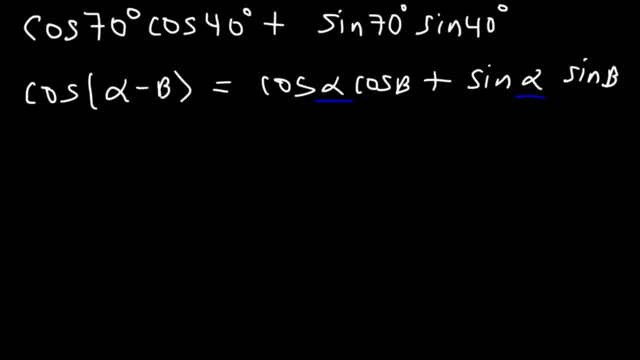 So we can see that Alpha is equal to 70 degrees And beta is 40 degrees. So we can't evaluate the right side. The right side is what we have here, But we can use the left side of the equation to get the answer. 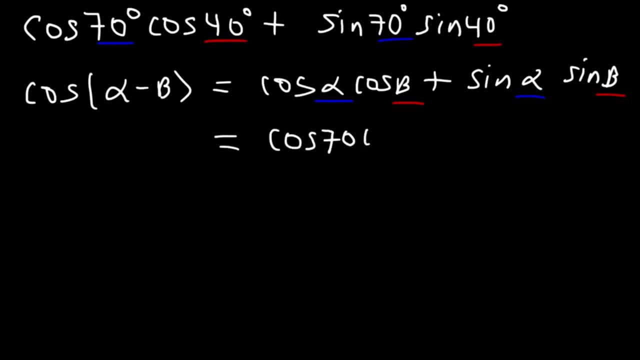 So therefore, cosine 70, cosine 40 plus sine, 70 times sine 40.. All of that Is equal to cosine alpha minus beta, or cosine 70 minus 40.. 70 minus 40 is 30.. So what we need to do is find the value of cosine 30, and cosine 30 is equal to the square root of three divided by two. 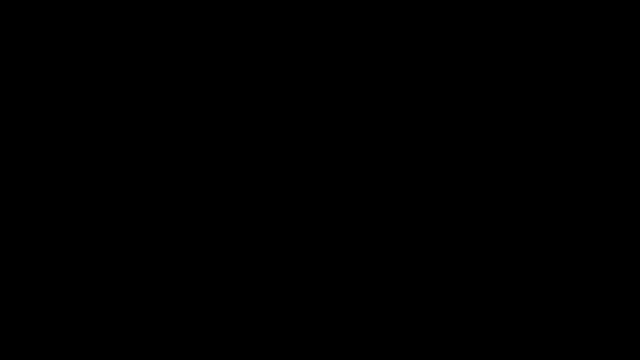 So this is the final answer. Now let's work on some more examples. Let's say, if we have cosine 20 times cosine 40. Minus Sine 20 times sine 40. Whenever you see two cosines together and two signs together, you know you're dealing with the sum of difference. formulas of cosine. 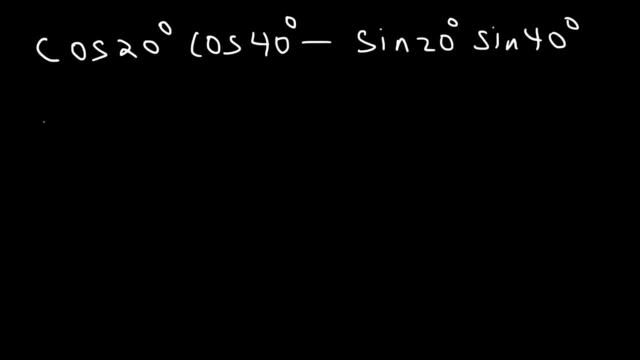 So notice that we have a negative sign with cosine. You got to reverse it, So this expression is equal to cosine alpha plus beta, where alpha is 20 and beta is 40.. 20 plus 40 and 40. Plus 20.. 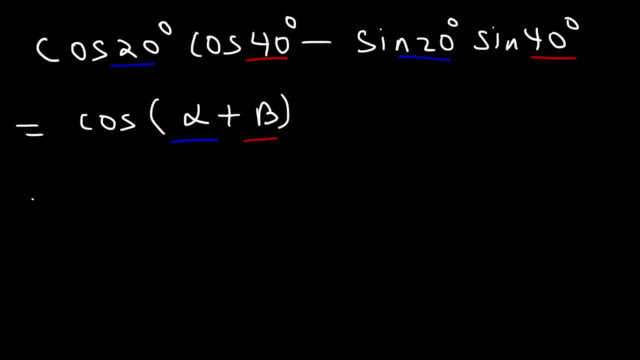 They both equal 60. So you just got to realize one of them is 21, of them is 40. The order really doesn't matter. So cosine 20 plus 40. That's equal to cosine of 60 degrees, and cosine 60 is one half. 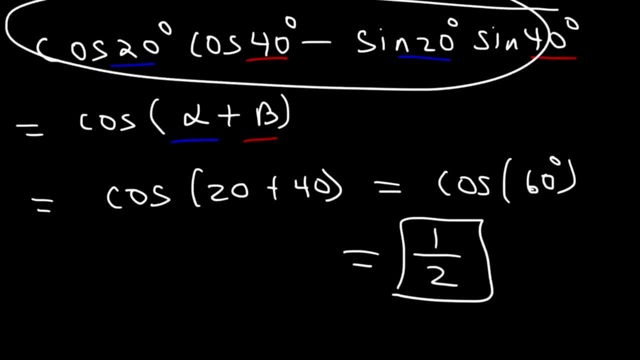 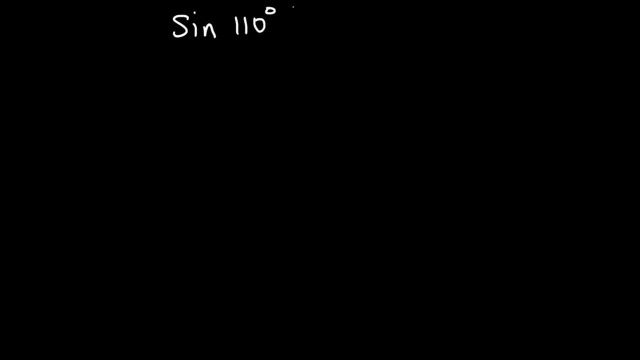 So that's the value of this entire expression. It's equal to one half. Here's another one: Sine of 110.. Multiplied by cosine 25.. Plus Cosine 110.. Times sine 25.. Go ahead and evaluate that expression. 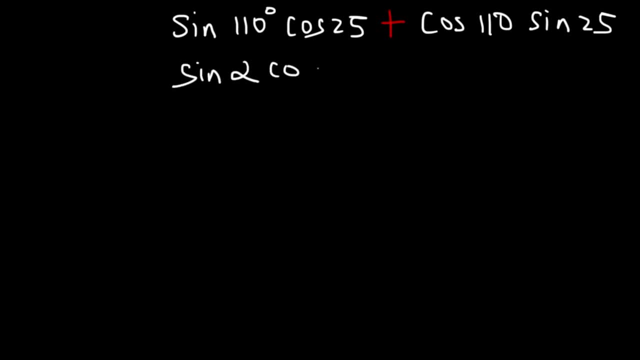 So we need to use this formula: Sine alpha, Cosine, beta plus cosine, alpha, sine, beta. So that is equal to the sine formula, And when dealing with sine, the sine doesn't change. So it's sine alpha plus beta. So we can see that alpha is 110 and beta is 25.. 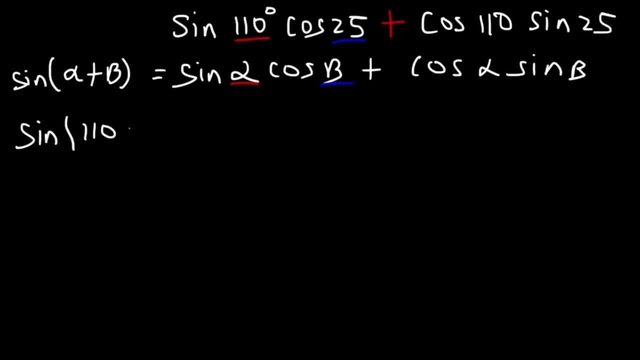 So then, this is going to be sine 110 plus 25. Which is sine of 135.. 135 is in quadrant 2. And it produces a reference angle of 45 degrees. Sine 45 is the square root of 2 over 2.. 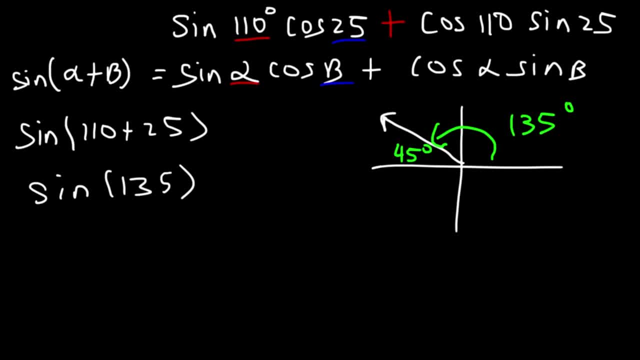 Sine 135 has the same value and it's positive in quadrant 2.. So this is going to be equal to the square root of 2 divided by 2.. And so that's the final answer for this entire expression. Let's try this one. 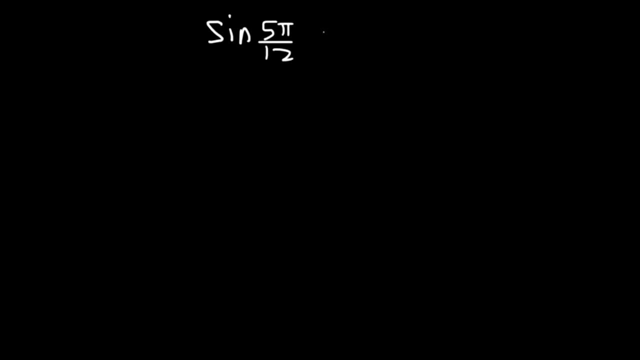 Sine 5 pi over 12.. Multiplied by cosine pi over 12.. Minus Cosine 5 pi over 12. Times sine pi divided by 12.. So whenever you see sine and cosine, You're dealing with the sum and difference formula of sine. 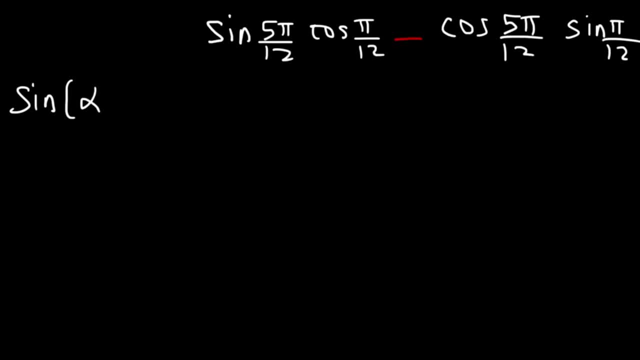 And since we have a minus sine, It's going to be sine alpha minus beta. So when you're dealing with a subtraction, The first one that you see here is alpha, Because the formula is sine alpha, Cosine beta, Minus cosine alpha. 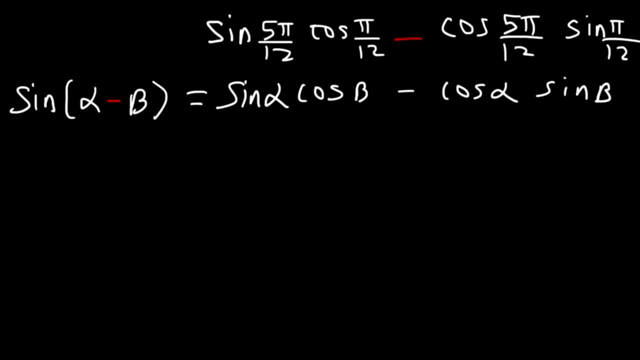 Sine beta. So you can clearly see that alpha Is 5 pi over 12.. Beta Is pi divided by 12.. So then this becomes sine 5 pi over 12.. Minus 1 pi over 12.. 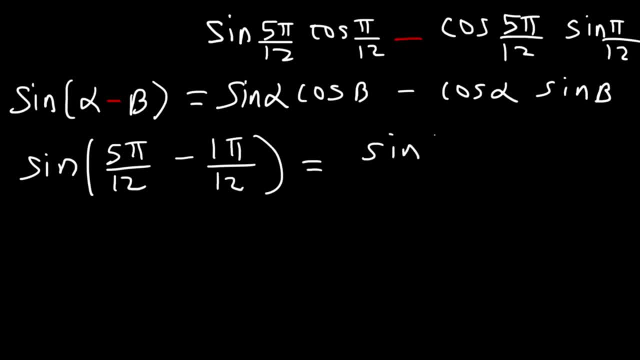 5 minus 1 is 4.. So now we have sine 4 pi over 12.. Now we can reduce 4 pi over 12.. 12 is 4 times 3. So we could cancel a 4.. So therefore we're looking for the value of sine pi divided by 3.. 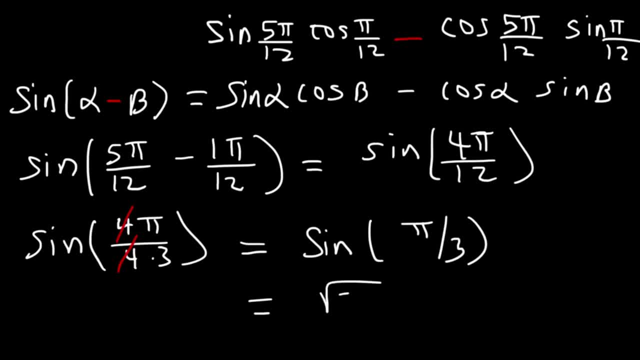 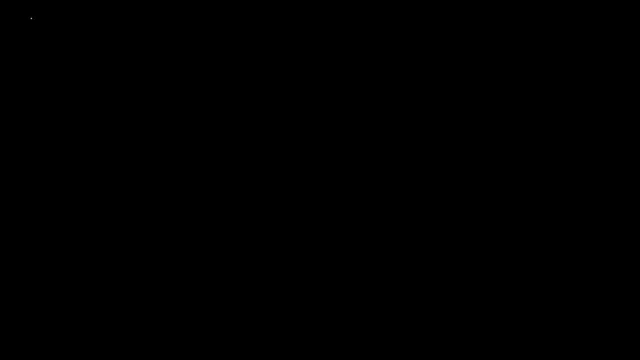 Pi over 3 is 60.. Sine of 60 degrees is equal to the square root of 3 divided by 2.. And so that's the final answer of the original expression. What is the value of tangent 15 degrees? So how can we get the answer for this problem? 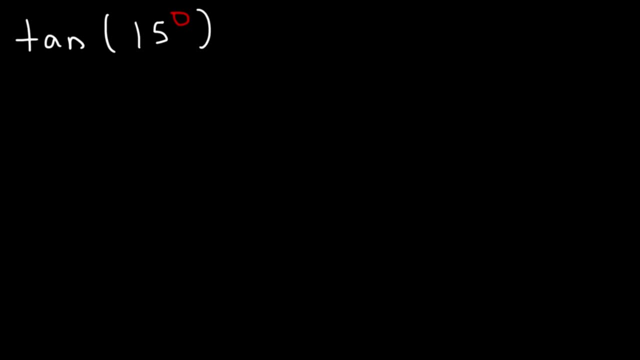 So first we need to find two angles that either add or subtract to 15. So let's use 60 minus 45. Now we need the right formula. Tangent alpha minus beta is equal to tangent alpha minus tangent beta. Tangent alpha minus tangent beta is equal to tangent alpha minus tangent beta divided by 1.. 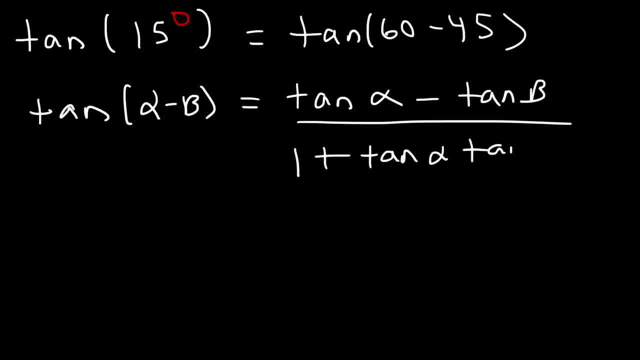 Plus Tan alpha, Tan, beta. So whatever sign you see here, this sign will be the same, But this sign here will change. Alpha is 60.. Beta is 45. So therefore, tangent 15, which is the same as tangent 60 minus 45.. 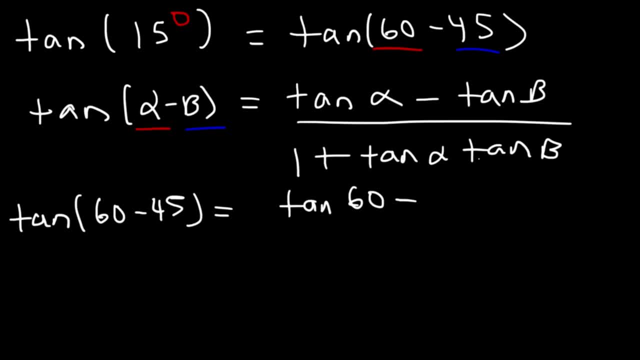 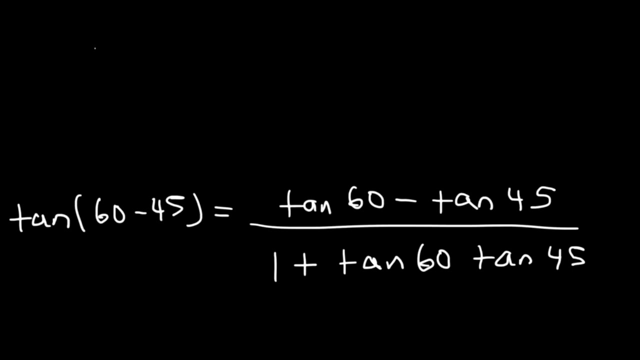 That's equal to tangent 5.. 60 degrees minus tangent of 45 degrees over 1, plus tangent 60 times tangent 45. Now what is the value of tangent 60?? Tangent 60 is equal to the square root of 3 and tangent 45 is 1.. And then we have 1 plus tan 60 times tan 45.. So this: 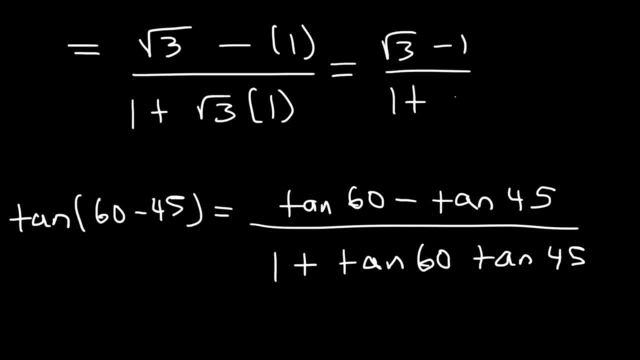 is the square root of 3 minus 1 over 1 plus the square root of 3.. So what can we do to simplify that expression? Whenever you have a radical on the bottom, you need to get rid of it. So what we need to do is multiply by the conjugate. 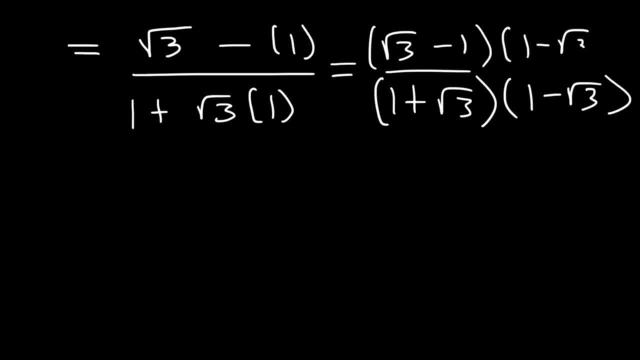 of 1 plus square root 3, which is 1 minus square root 3.. So let's FOIL. Here. we have the square root of 3 times 1, and that's simply square root 3.. And then the square root of 3 times itself, that's the square root of 9,, which is 3.. And then 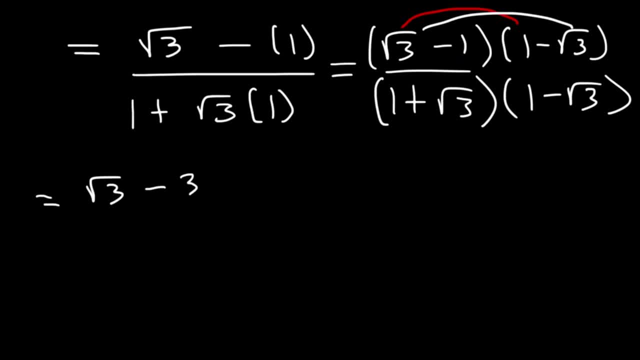 you have the negative sign. Next we have negative 1 times 1,, that's simply negative, 1.. And then negative 1 times negative, square root 3,, which is positive square root 3.. On the bottom, first we have 1 times 1,, which is 1.. And then 1 times negative. 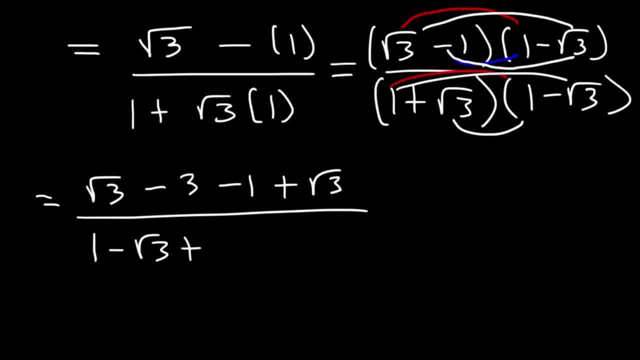 square root 3.. And then positive square root 3 times 1.. And then square root 3 times negative square root 3, which is negative, square root 9, and that's 3.. On the bottom, these two terms will cancel. On top we can add the square root of 3 plus the square root of 3,. 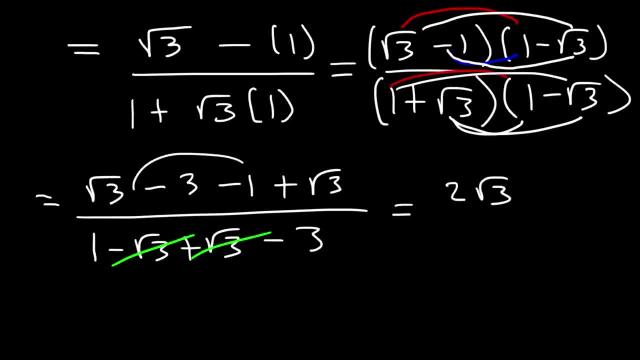 which is 3.. 2 square root, 3. Negative: 3 minus 1 is negative 4.. 1 minus 3, that's negative 2.. So now what we're going to do is we're going to divide 2 square root 3 by: